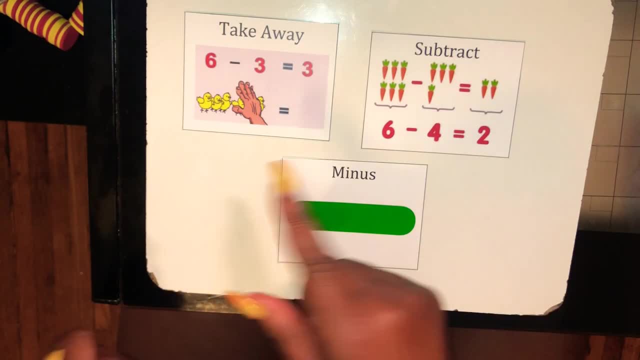 it means to cross out some or get rid of some. Subtraction means the same as takeaway. It's just another way to say takeaway, And minus is the sign that we use when we're doing subtraction. All right, boys and girls, let's get started. So I have a little problem I'm going to solve. 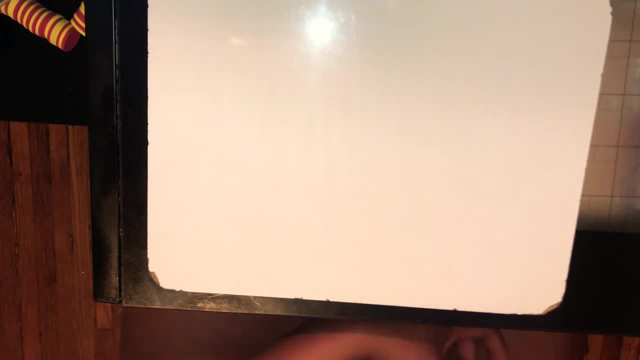 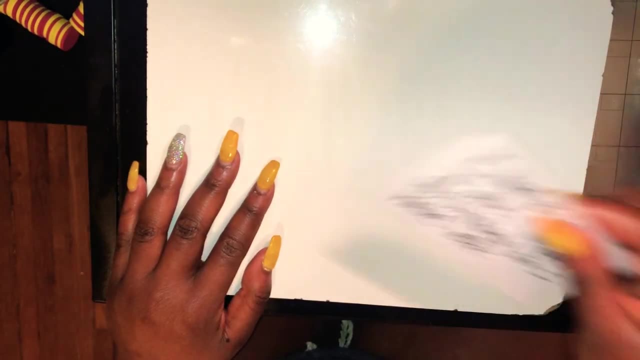 all by myself. And then you guys are going to help me to solve another one. I had eight lollipops. I ate one lollipop. How many lollipops do I have left? So watch how I solve this. I have eight lollipops. I ate one lollipop. How many lollipops do I have left? 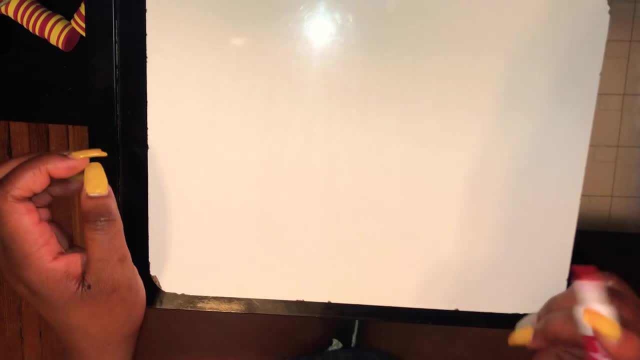 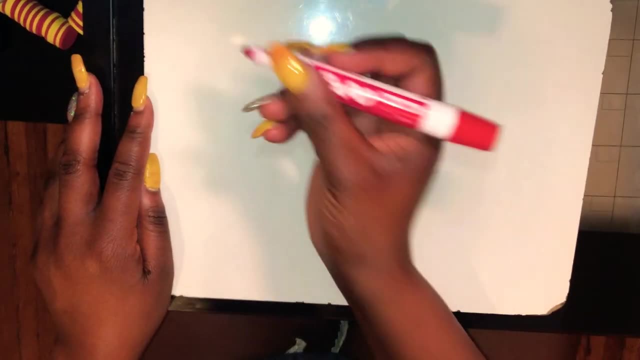 So watch how I solve this problem. I'm going to draw a picture and then I'm going to use my manipulatives. So first, how many lollipops did I have all together? Oh, I had eight, So let's draw. 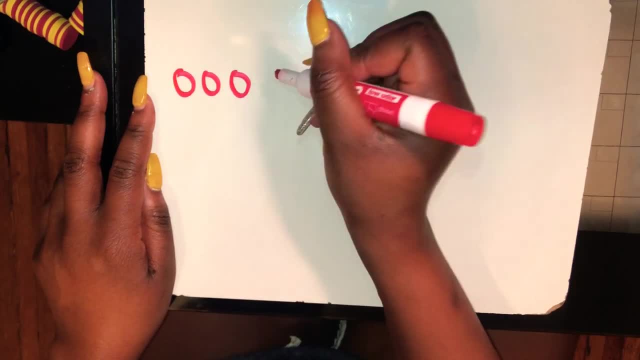 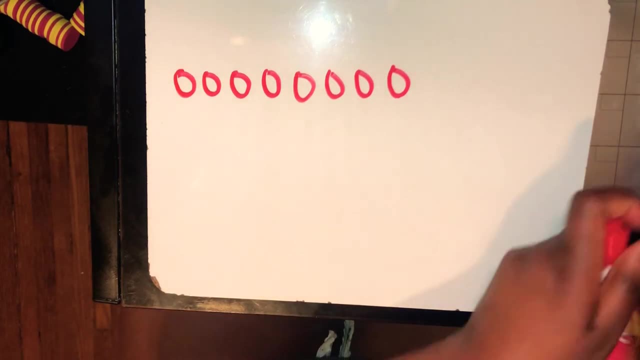 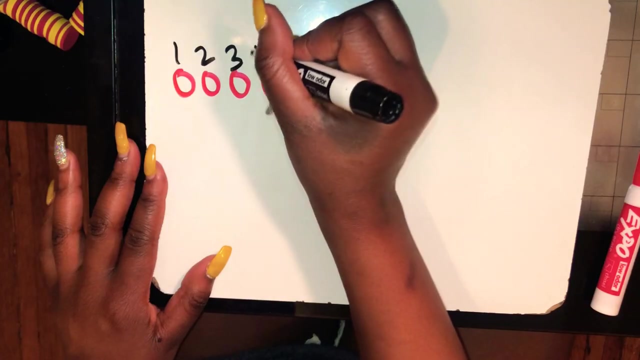 eight circles: One, two, three, four, five, six, seven, eight. I had eight lollipops, And so I don't get confused. I'm going to write the number right on top, That's one, two, three, four. 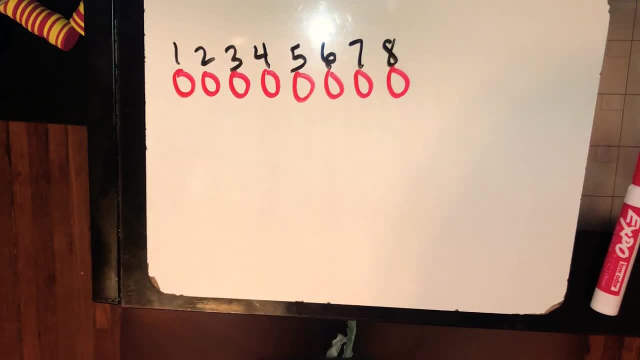 five, six, seven, eight. I have eight lollipops. Now what happened? I ate one, I ate one. So if I ate one lollipop, does that mean I get another lollipop or I get rid of it? Yeah, When you eat. 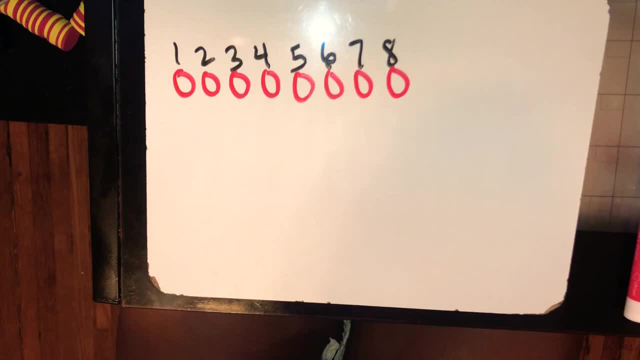 something it goes away. So I had ate one lollipop, So I'm going to cross out one lollipop. Now I need to figure out how many lollipops I have left. To figure out how many lollipops. 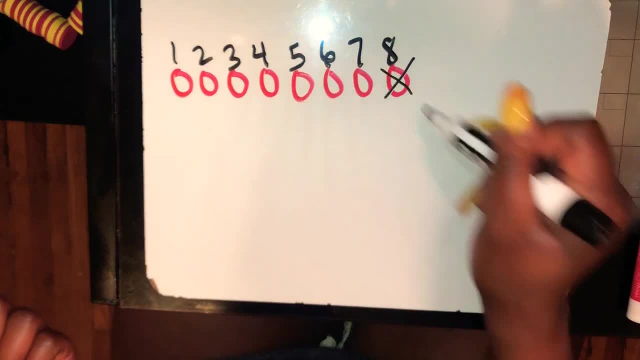 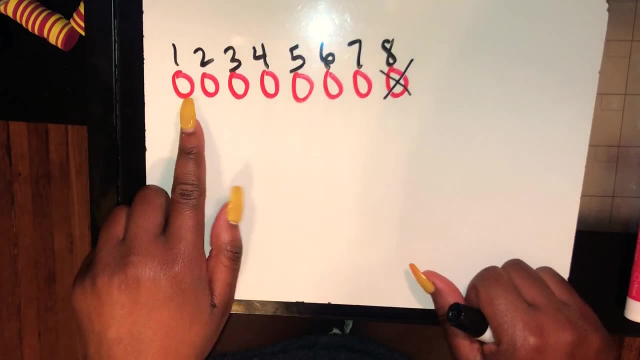 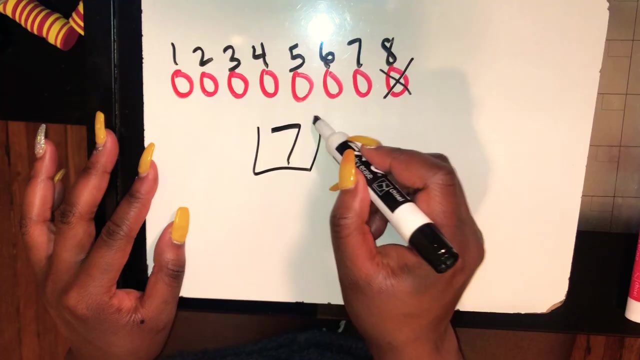 I have left. I have to count how many are left after I crossed out the one that I ate. I don't really have to count because I already wrote all the numbers, but I'm going to count just to be sure. One, two, three, four, five, six, seven. Oh, I have seven lollipops left. 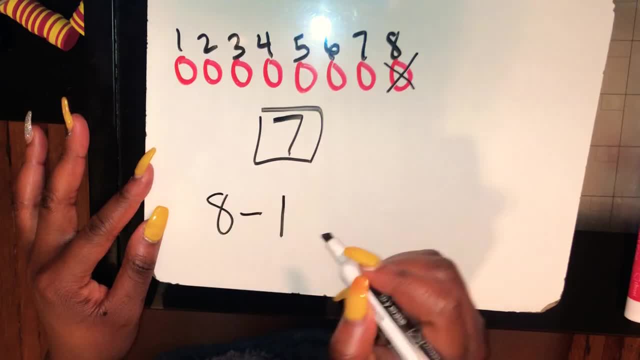 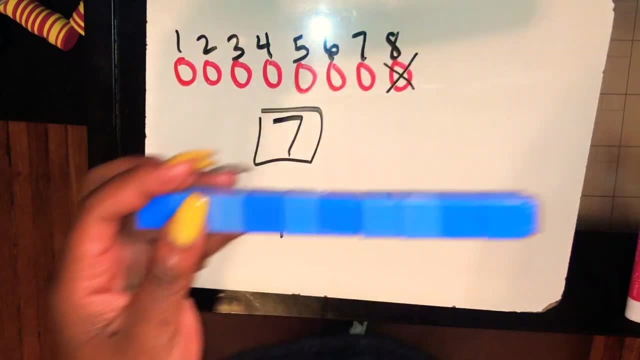 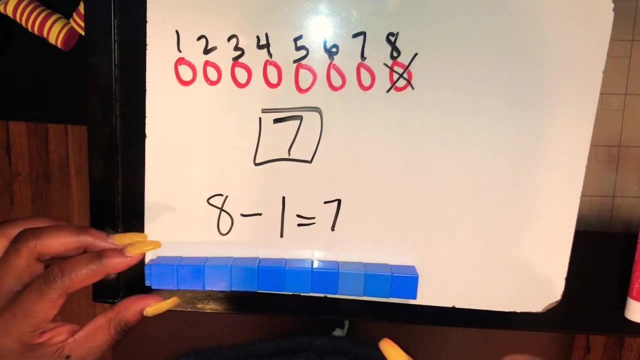 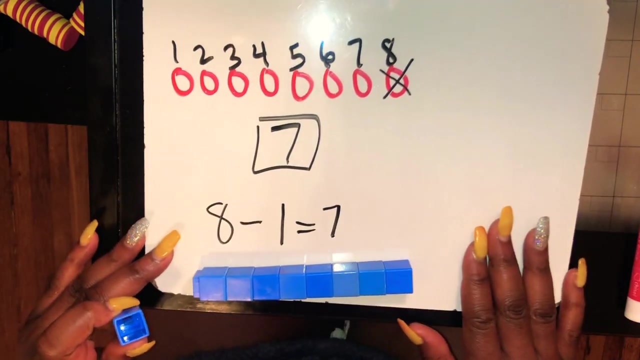 Another way that I could write that is: eight take away one equals seven. All right, I just want to use my cubes to help me show: eight, take away one. So how many lollipops did I have first? Yep, I had eight. So let's count: eight, One, two, three, four, five, six, seven, eight. I had eight lollipops. 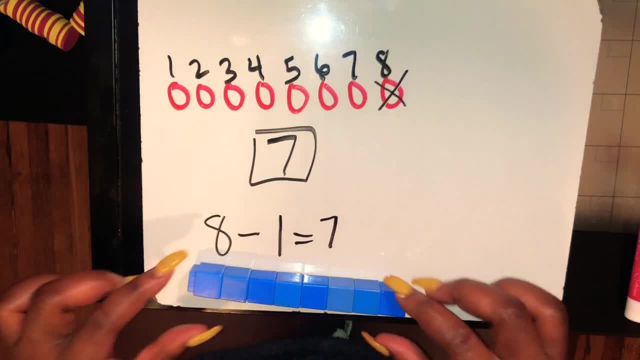 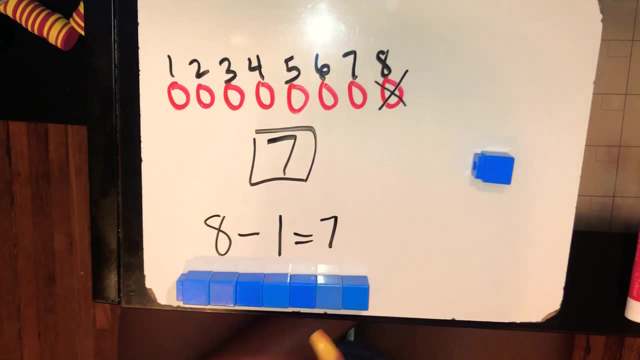 Now what happened? Oh, I ate one, So I'm going to take away one of my lollipop because I ate one. Now I'm going to count to see how many I have left: One, two, three, four, five, six, seven, Yeah, 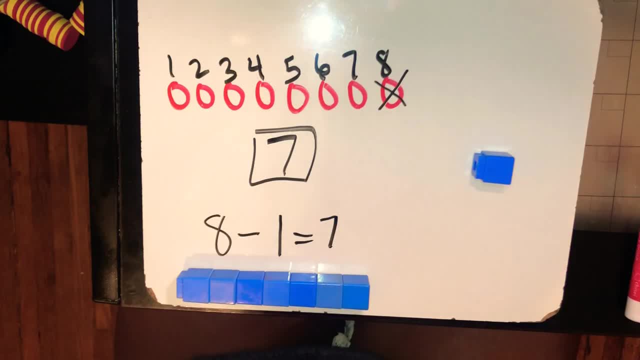 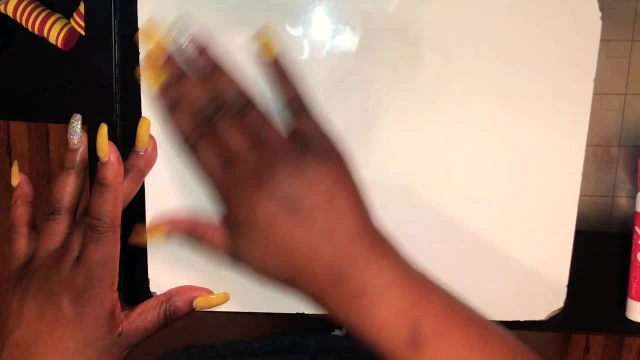 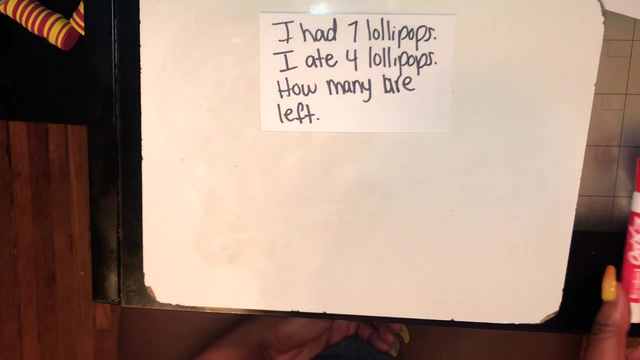 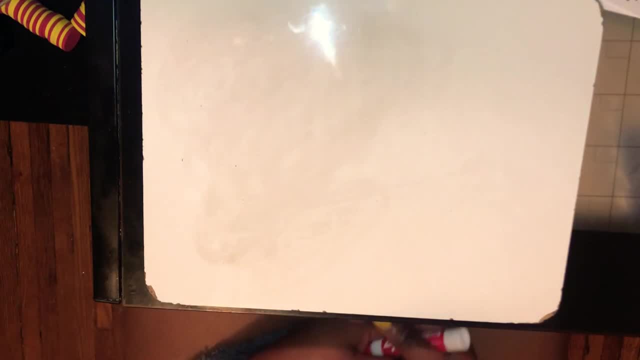 many lollipops are left, So let's think about it. I had seven lollipops. How many should I draw? Yeah, I'm going to draw seven. Can you draw seven on your board? And I'm going to draw seven, right. 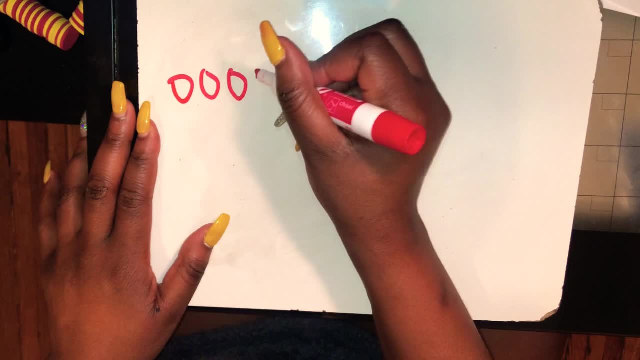 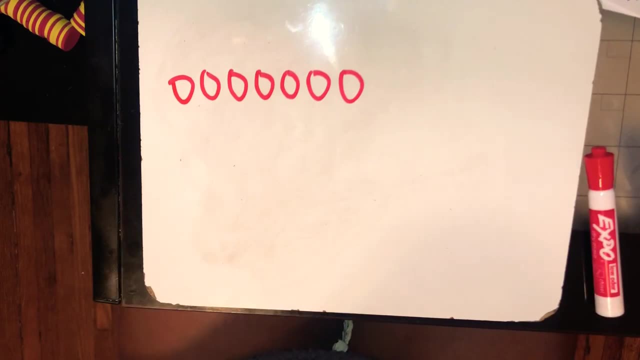 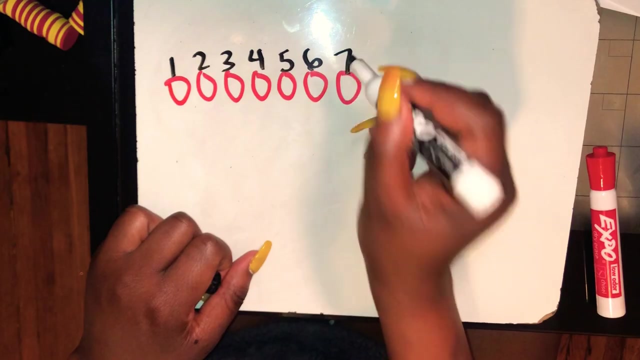 here: One, two, three, four, five, six, seven. Yep, I drew seven lollipops because I had seven to begin with, And I'm going to write the numbers on top so I don't get confused. I had seven lollipops, And then what happened? I ate four. I ate four lollipops, So let's count. seven lollipops left. I ate four lollipops. How many lollipops? I had eight lollipops. How many lollipops left? I had eight lollipops. How many lollipops left? Seven lollipops. How many lollipops? 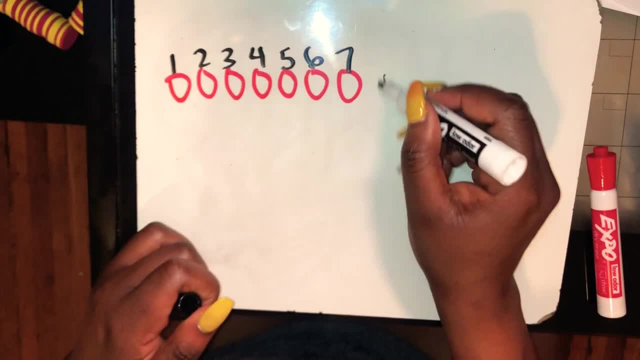 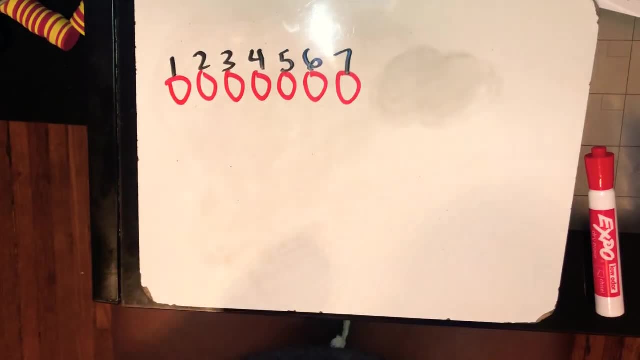 lollipops. So what should I do? Should I draw plus four lollipops or should I cross some out? You're right, I'm going to cross some out, because if I ate the lollipops, they're gone. They're no. 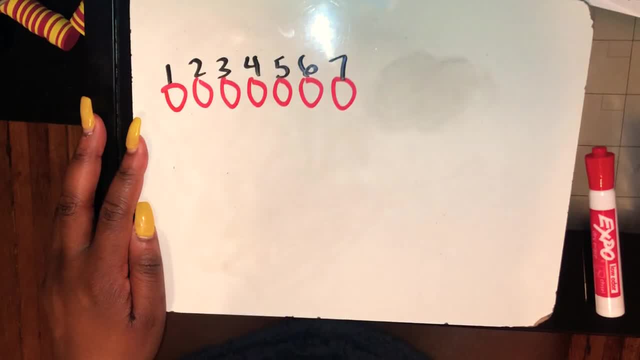 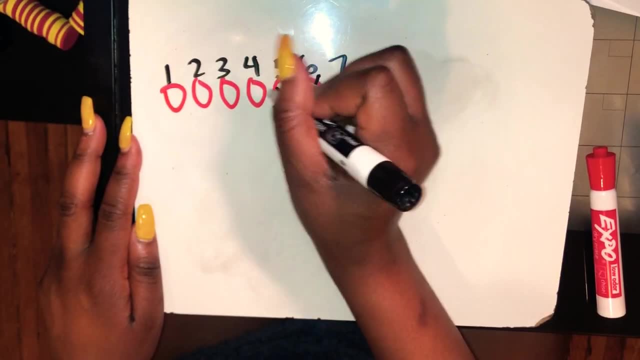 more, So I need to get rid of them. So I had seven lollipops and I ate four. Let's cross out four together. Let's count One, two, three, four. So I crossed out four lollipops. How many do I have? 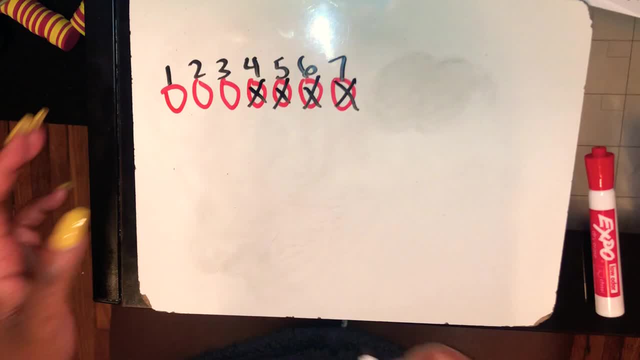 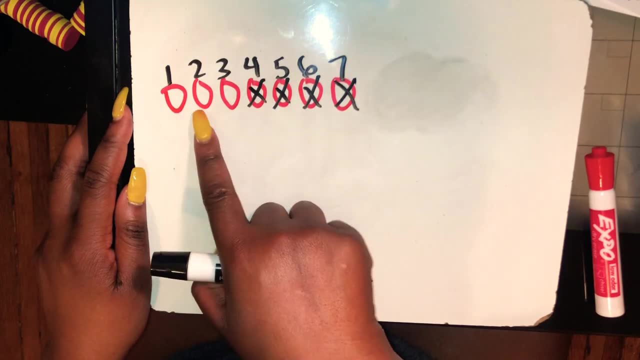 left. now, Yep, I cross it out and then I count. So I drew seven lollipops, I crossed out four. Now I need to count to see how much I have left. One, two, three. I have three lollipops left. 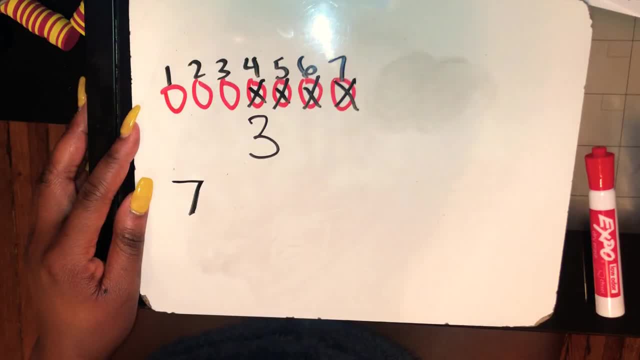 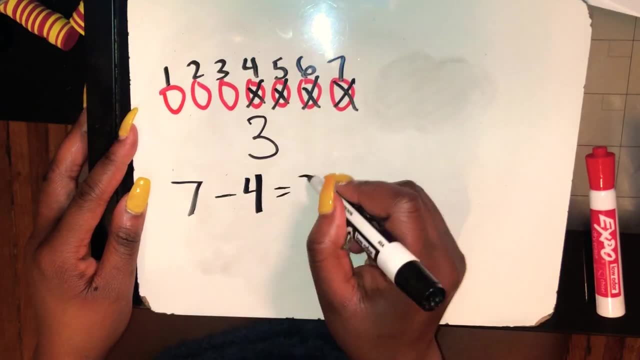 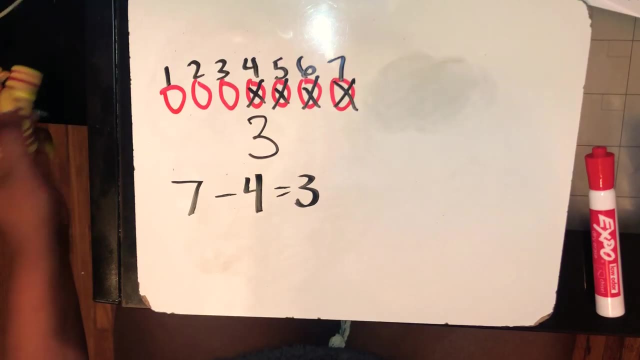 Another way that I can write that is: I had seven lollipops when I started the minus sign. because this is a subtraction problem, I took away four and now I have three. I'm going to use my counters to show you how I do this, because I did this for my cubes, So now I want to try a. 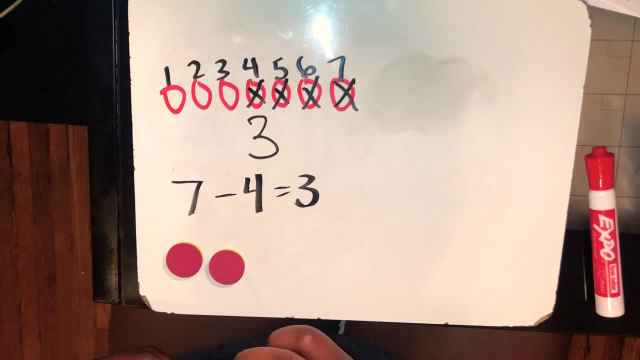 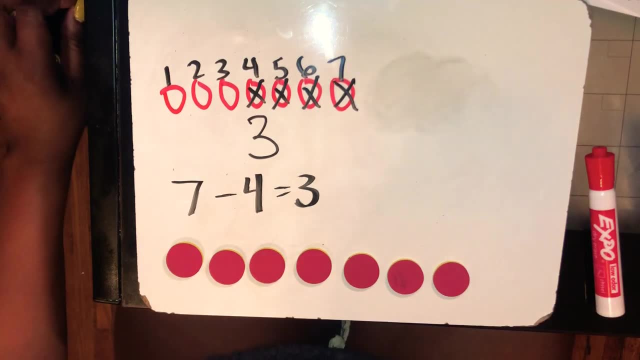 different strategy, different manipulative: One, two, three, four, five, six, seven. So I had seven lollipops: One, two, three, four, five, six, seven. Then what happened? Yep, I ate four. So I'm not going to cross it out because I have manipulatives, I'm just going to 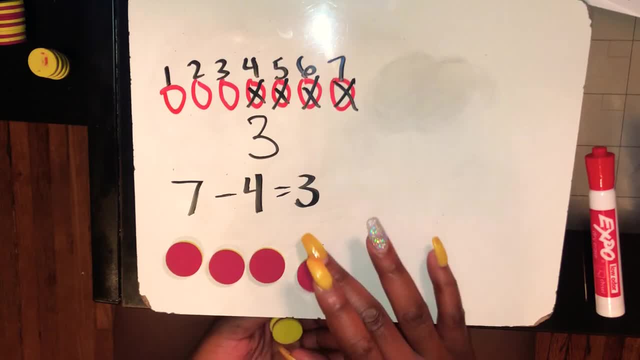 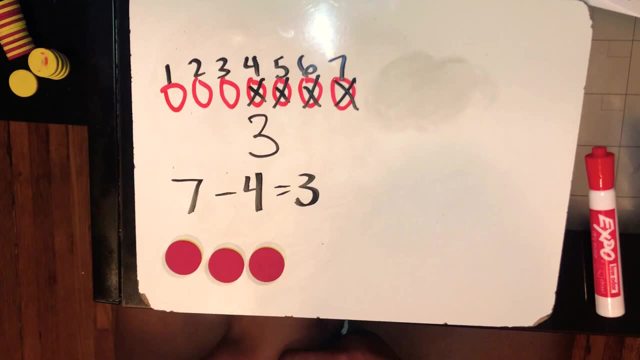 take them away. One, two, three, four. How many do I have left? Three, because seven. take away four equals three. All right, boys and girls, Now let's try one. You're going to try one by yourself, and then. 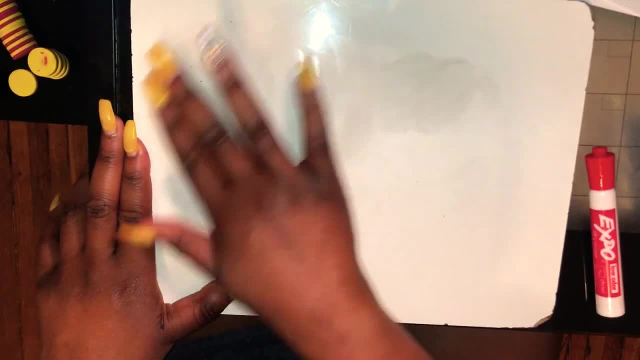 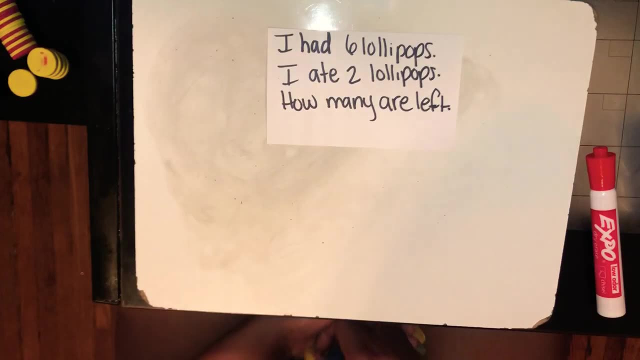 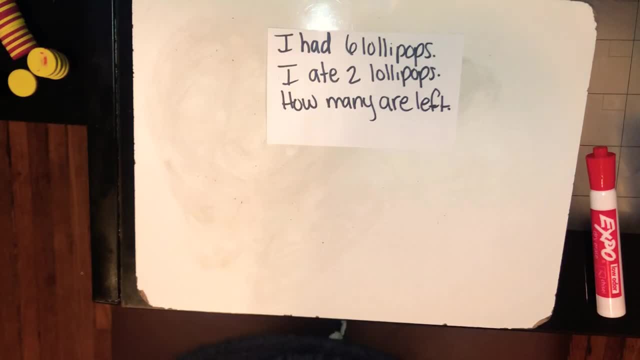 I ate two lollipops. How many lollipops are left? I want you to draw a picture to show this. So I had six lollipops. I ate two of those lollipops. How many lollipops do I have? 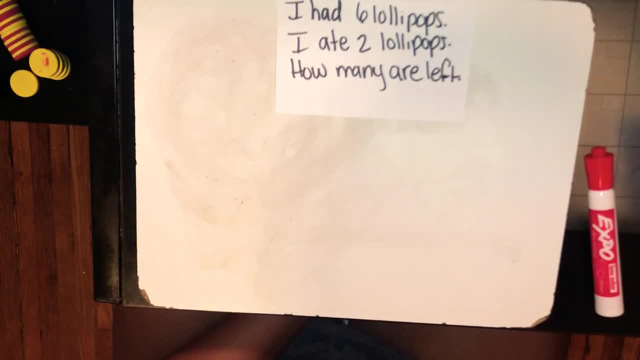 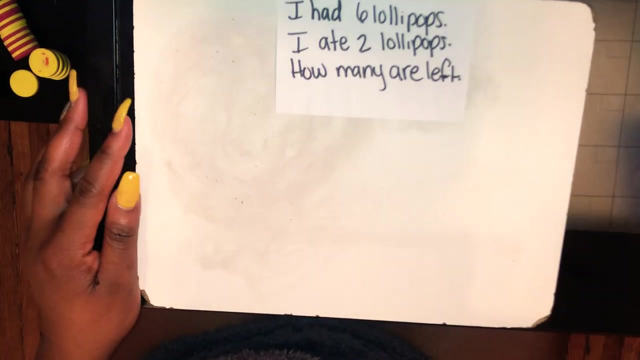 left. Try and solve it. I had six lollipops. I ate two lollipops. How many are left? Okay, now let's check your work. So how many lollipops should I draw? Did you say six? Yep, because I had six lollipops when I started One. 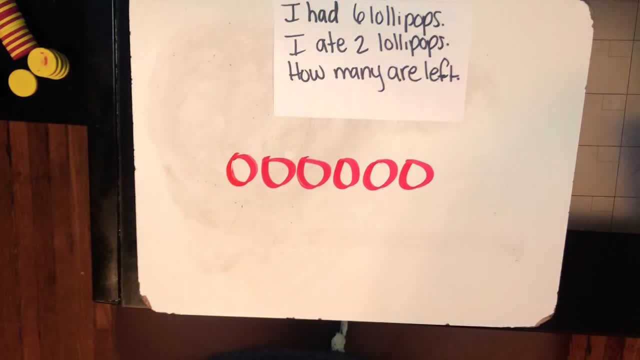 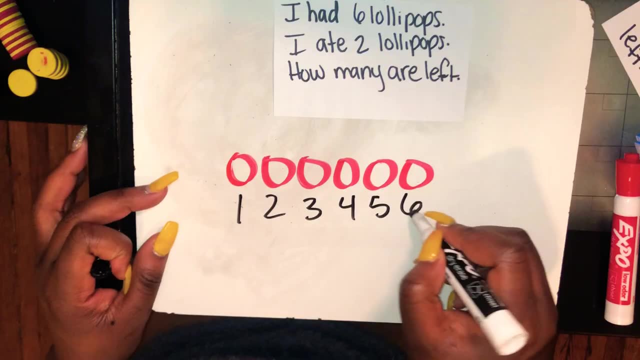 two, three, four, five, six. And just so I don't get confused, I'm going to write the numbers underneath: That's one, two, three, four, five, six. So I have six lollipops. Then what happened? 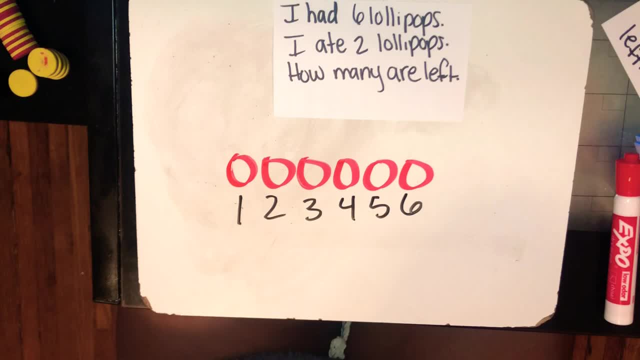 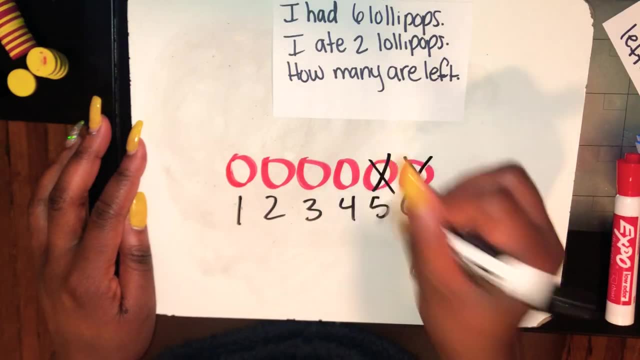 Did you say I ate two. So what should I do if I ate two lollipops? Mm-hmm, Did you cross out two lollipops, And how many do we have left? Let's count One, two, three, four, five, six. And just so I don't get confused, I'm going to write the numbers underneath.